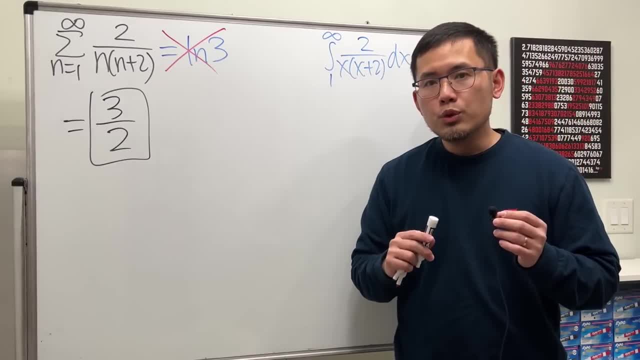 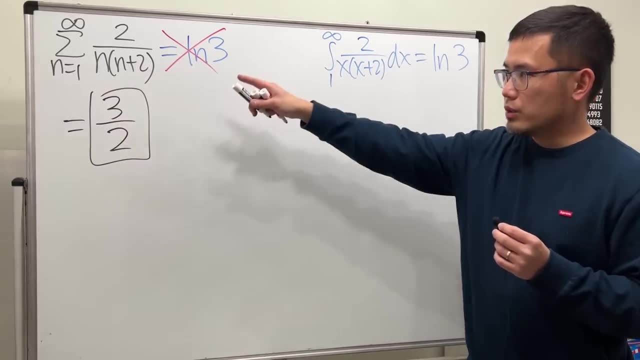 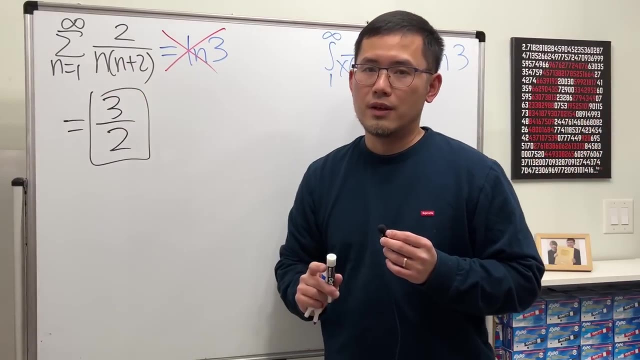 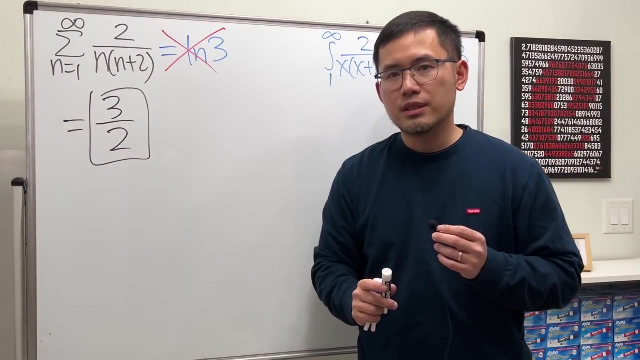 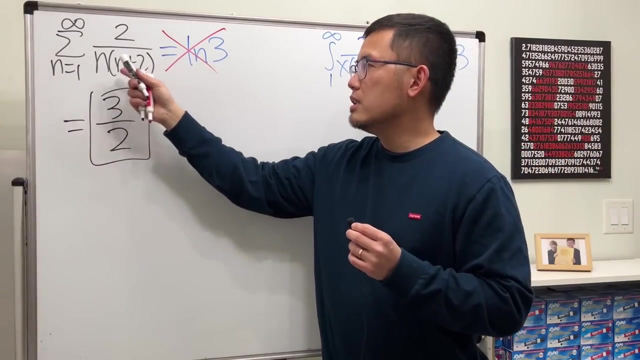 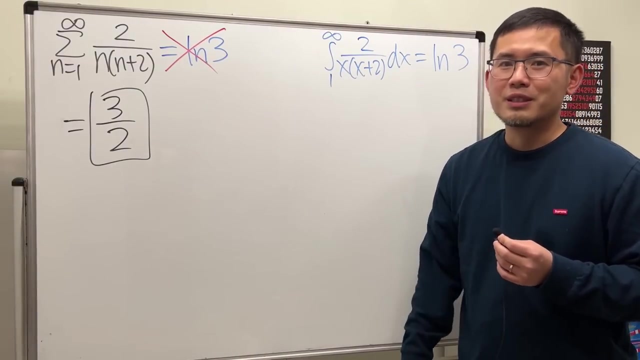 So here is what we have to be careful When we use the integral test. what we can say is the following: If this corresponding improper integral to the infinite series, if this right here converges, then we can come in and say: this right here also converges. Likewise, if this right here diverges, then this right here also diverges. One thing that we cannot say is that if this right here is equal to ln3, do not come in and say this right here is equal to ln3 as well. They will not converge to the same value, except for some very famous questions. 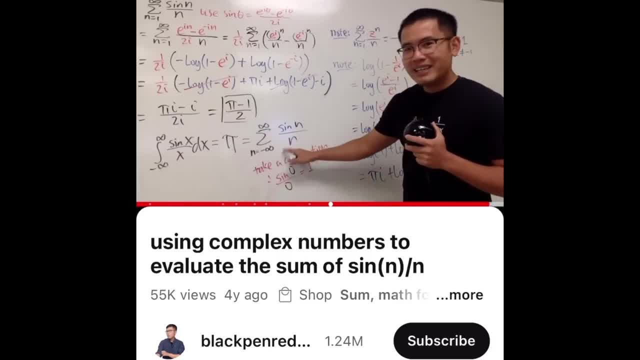 This improper integral is the same as the infinite series, this infinite series and both of them. magically, they're equal to pi. just amazing. if this is not amazing, i don't know what it is. you can check one out in the description, but in this case they are. 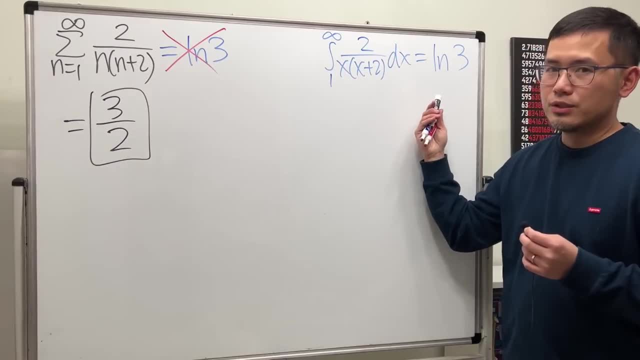 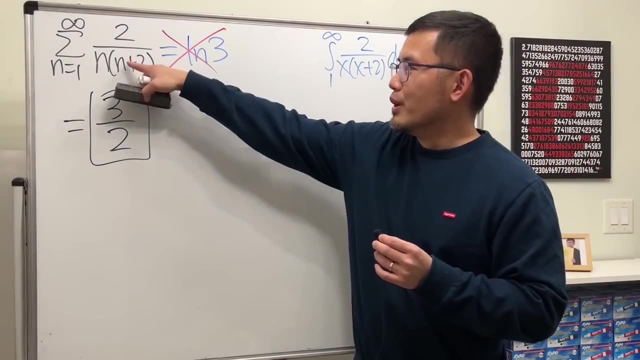 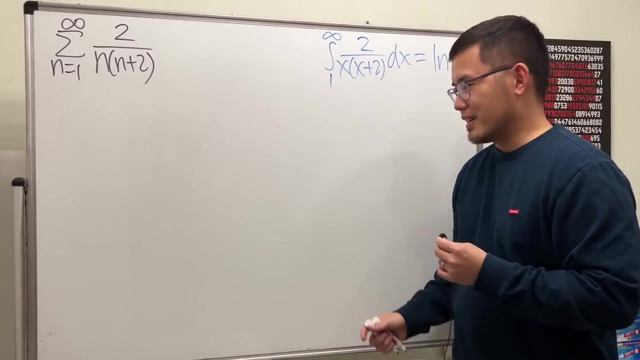 not, this is 3 over 2, this is ln 3, right? so hopefully this right here is clear. that's it. of course not. i will, of course, show you how to go from here to here, how to get that 3 over 2, and i'm going to leave the improper integral to you, okay, so here we go. originally the denominator. 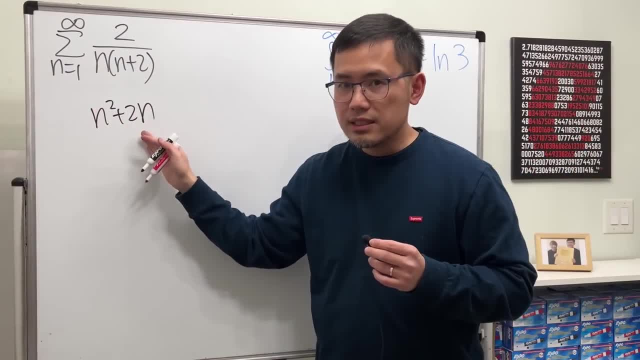 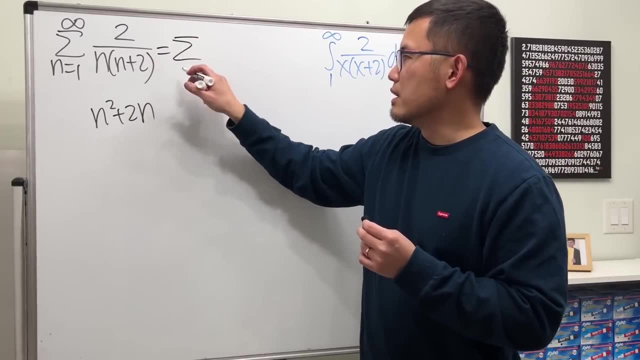 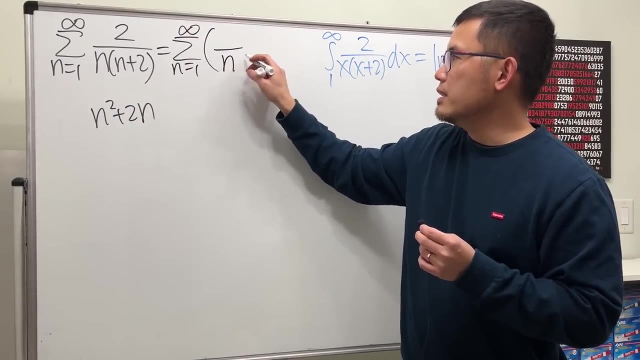 was given to be n squared plus 2n. if that's the case, make sure you just factor it so that we can do partial fractions. so this will be here. we have the series as n goes from 1 to infinity. we have n right here. so that means we have some number over n plus n plus 2 for the second. 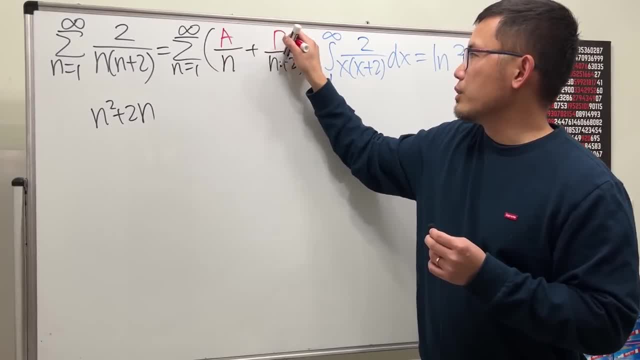 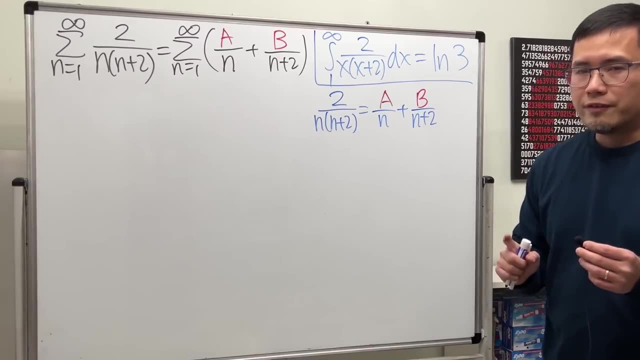 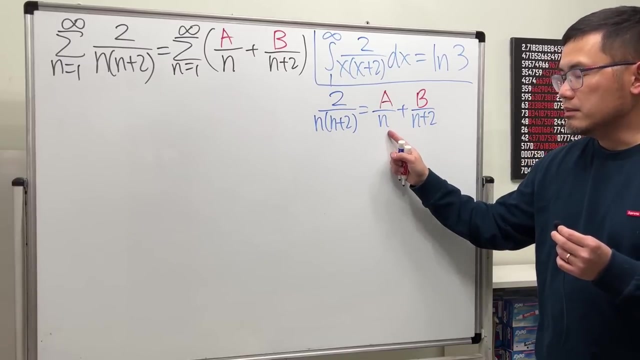 denominator. all right, let's call this a and let's call this b, and of course, we will have to figure out what a and b are. i will show you the fast way first, and then i will explain why the fast way works. the fast way is the following: we have a over n. we are going to cover the denominator from the. 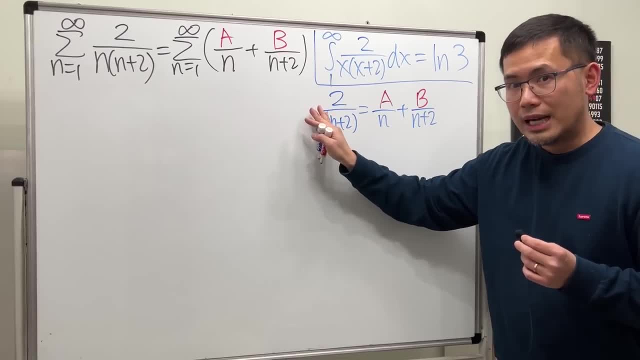 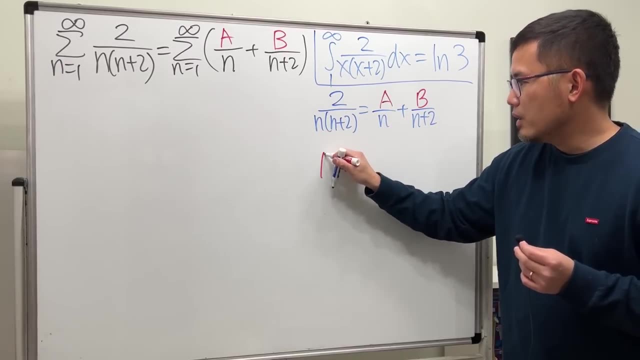 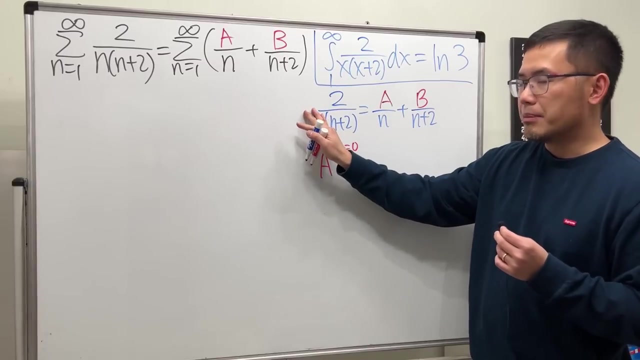 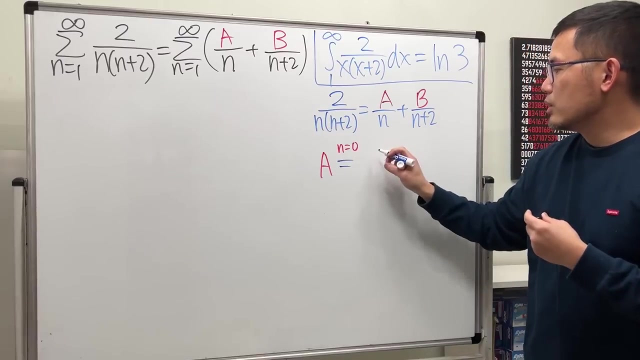 original the same denominator n, and you ask yourself: how can we make this n equal to zero and just equal to zero? so a will be equal to. we make n equal to zero. but remember we covered this up- we are going to put this n equal to zero into this n. this is the only remaining n, so we get 2 over 0 plus 2. work that. 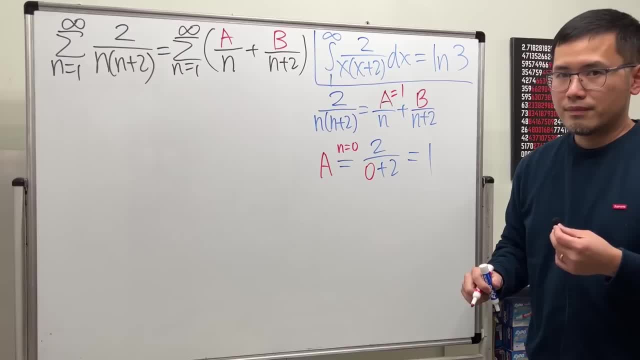 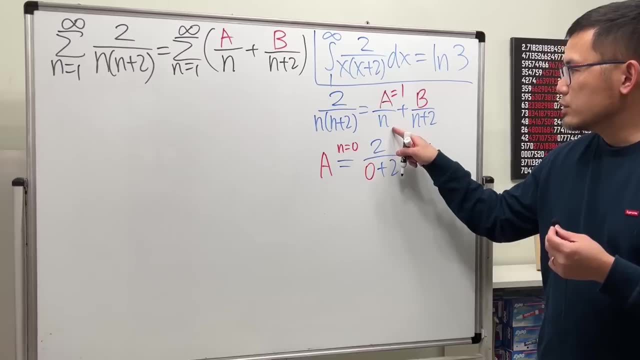 out, we get 1, a equals 1. this, right here, is called the cover-up method and just real quick, let me show you why it works. as we can see, we have a number over n plus 2 and we have a over n plus 2. 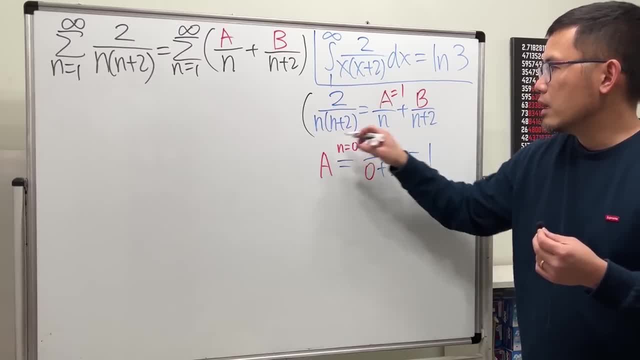 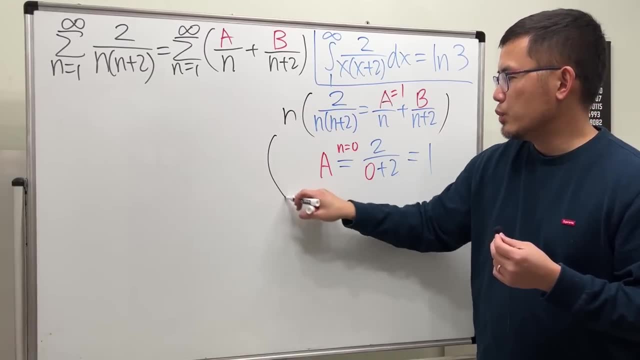 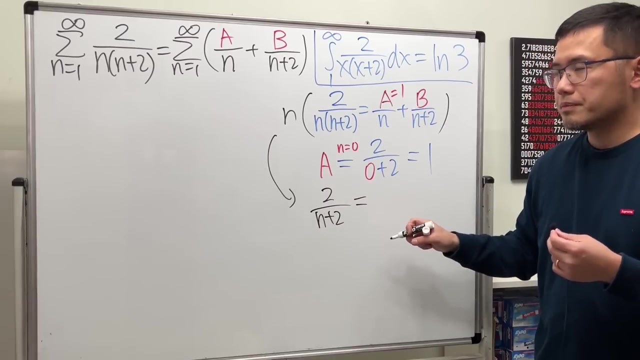 we have n for the denominator, like for the a. instead of multiplying everything by this and that, let's just multiply everybody by n, and then we will get the following: we will get 2 over n and n cancel. so just n plus 2, that's equal to n and n cancel. so we just get a and then this times that. 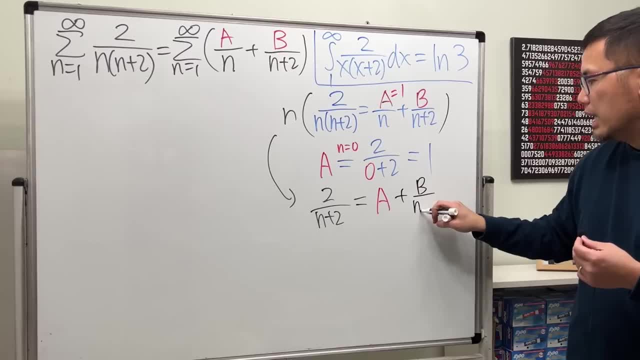 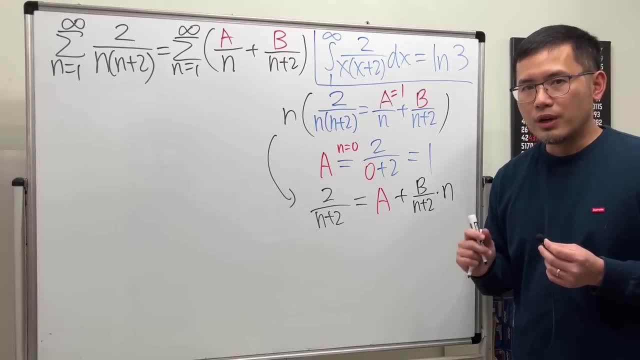 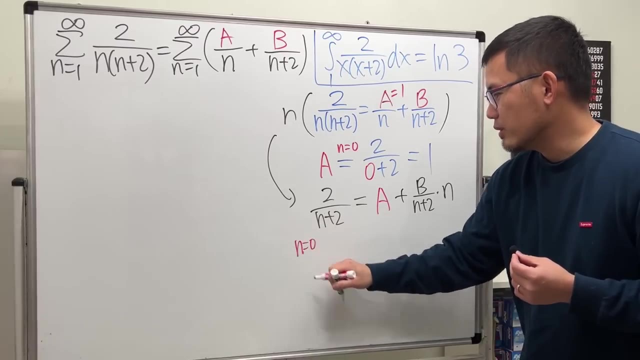 nothing cancels. so we will have b over n plus 2 times n. now look at this equation. let's pick a very nice number for n to get rid of this term. what number? zero. yes, let's put n equal to zero, because this way, you will see, we get 2 over 0 plus 2. 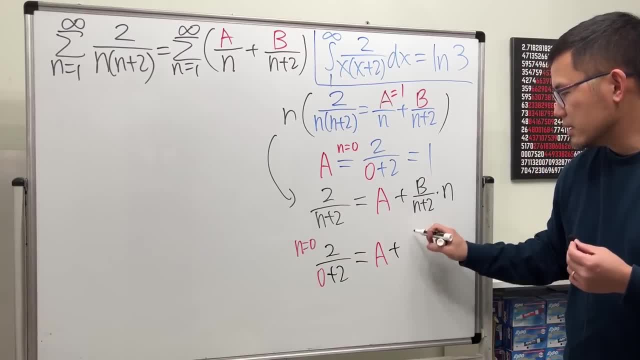 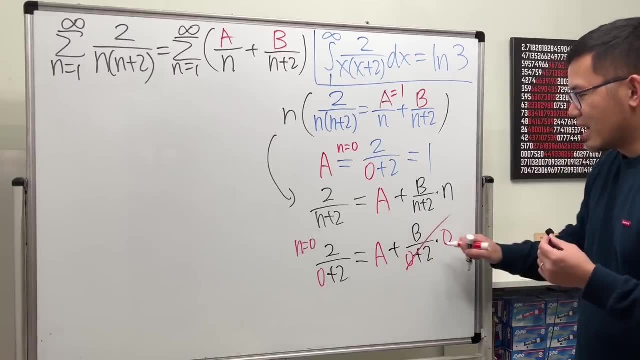 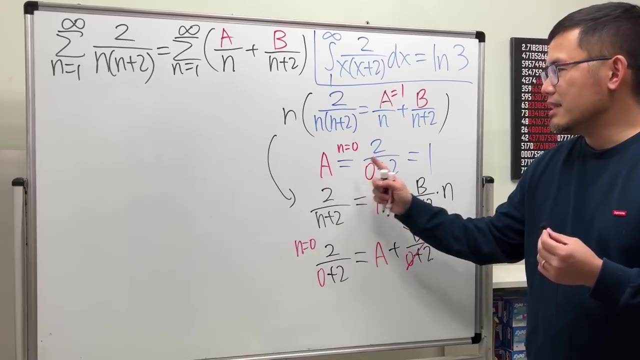 that will be equal to a plus b over 0 plus 2 times zero. of course, this term is gone. you don't have to worry about b. a equals 2 over 0 plus 2. that is exactly what i showed you, so now let's use the cover method. 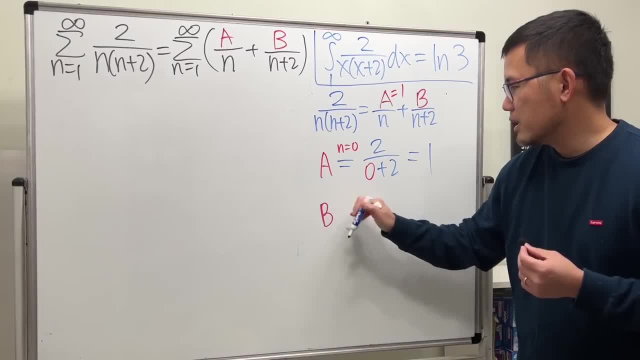 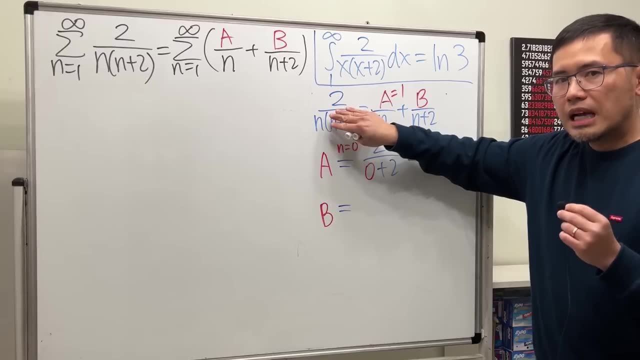 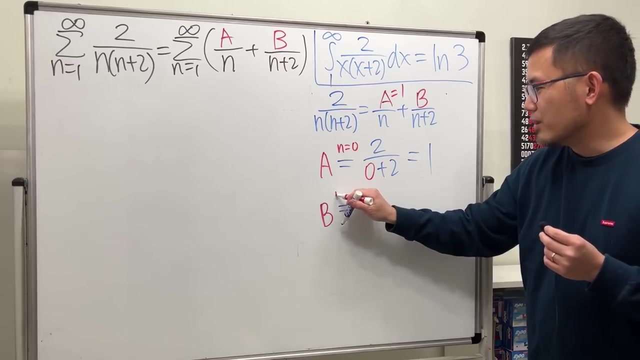 to figure out what b is b? okay, it has the denominator n plus 2. we come here cover this up. in the meantime, you ask yourself: how can we make n plus 2 equal to 0? n has to be negative 2, so pick negative 2, and then we are going to do the following. we are going to do the following: 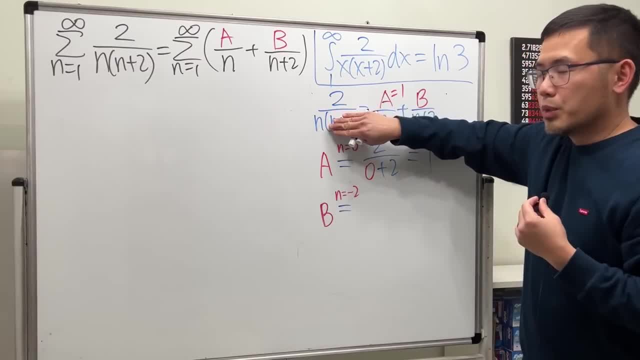 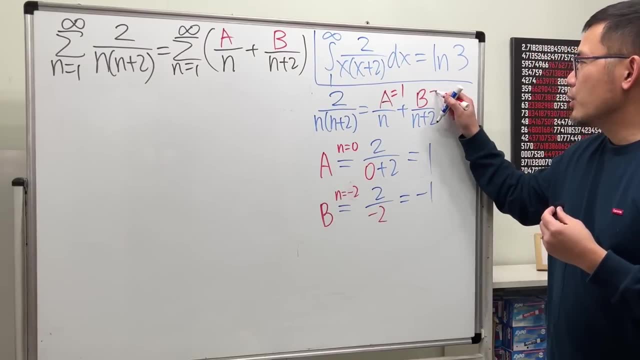 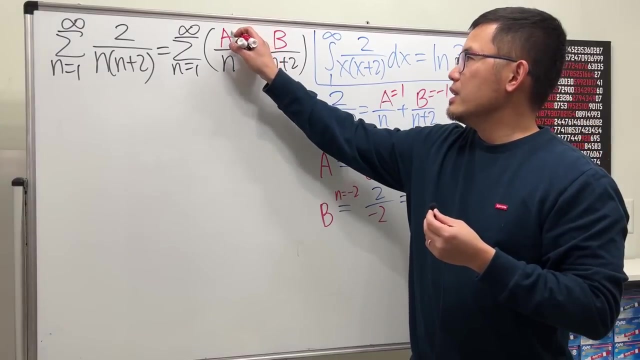 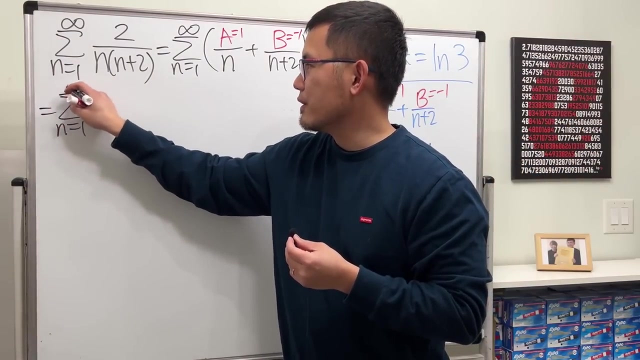 we are going to put the negative 2 into this n. this is capital l already, so we have 2 over negative 2, which is just negative 1. so b equals negative 1. it works wonders. so now we can just come back here: a equals 1, b equals negative 1. so this means we have the series as n goes from 1 to infinity of. 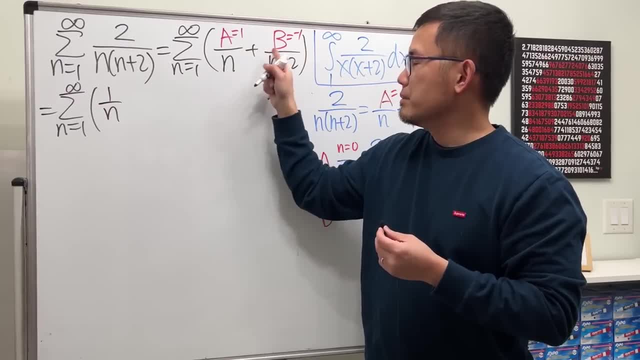 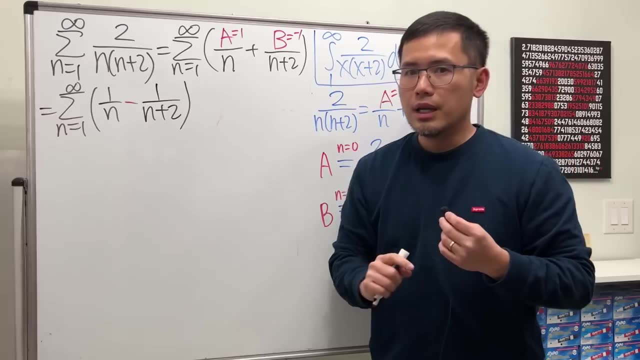 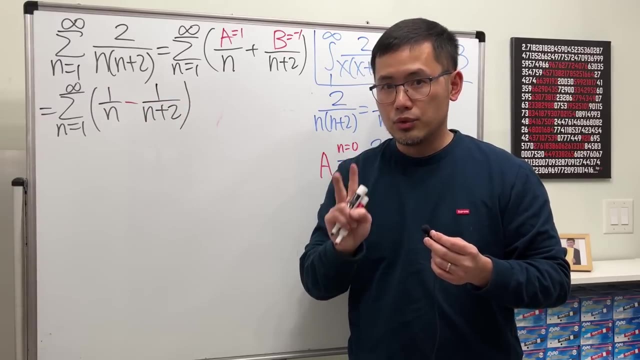 1 over n minus. right, because this times that's minus 1 over n plus 2. now here's the deal. notice that we have a subtraction and the first term here and this term right here. they are all by 2. what i mean by that is the. 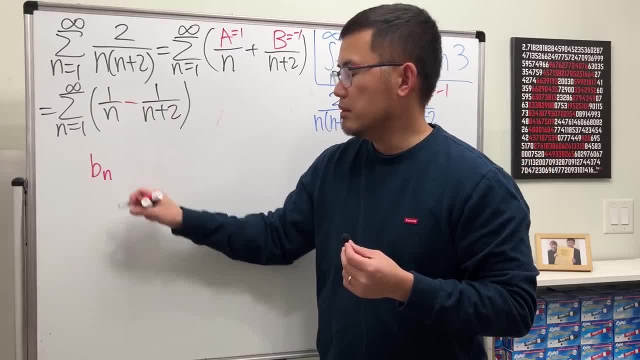 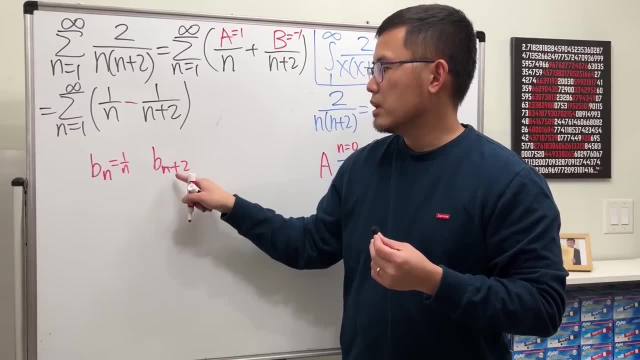 following this right here. if you look at this as b n, then this right here is just b sub n plus 2, right? if b? n is equal to 1 over n, b sub n plus 2, you just put n plus 2 into this n. 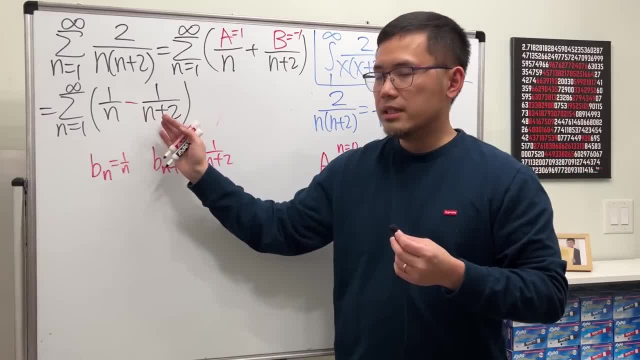 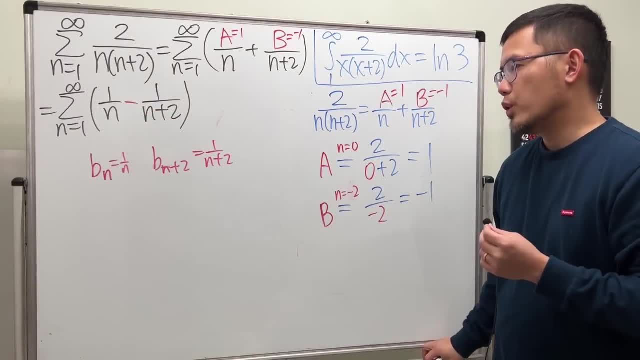 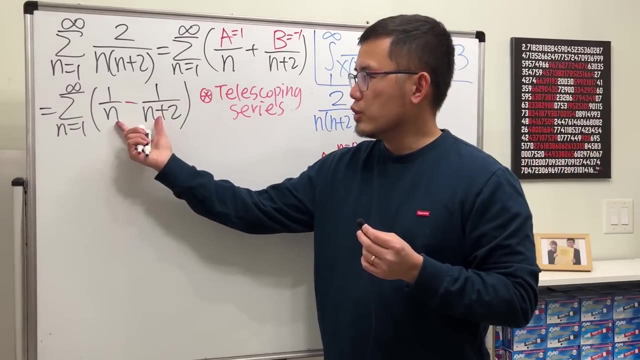 2 over n plus 1.. So this and that are pretty much the same kind, but they are just all by 2 and we have a subtraction. in this case, we will get a telescoping series. So how do you proceed, though? we are just going to write down several terms for this and you 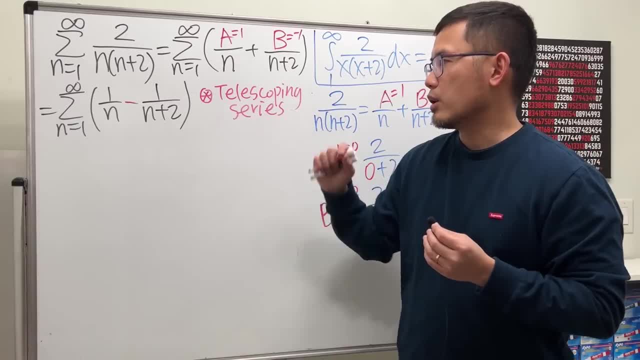 will see that a lot of times we can, so that's why it's called the telescoping series. so let me show you first. leave a space right here, okay, let's get started. first. let's Farmzen série n en auto. So let me show you first. leave a space right here, okay, let's get started. 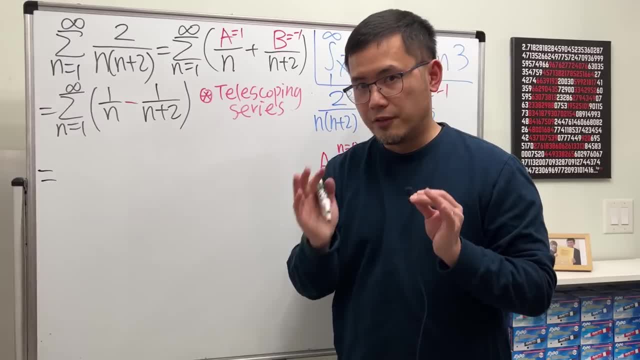 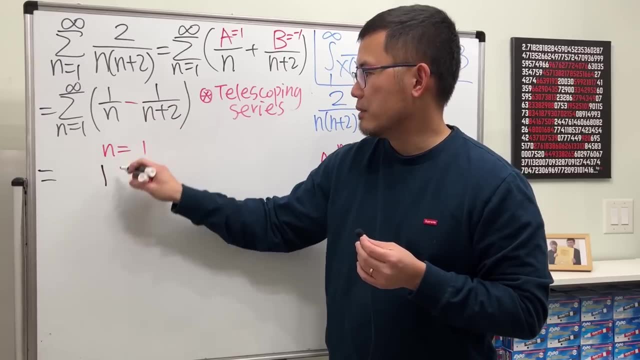 right here. okay, let's get started right here. let's get started right here. let's get started. go ahead and plug in 1 into this n and that n for the first term. so when n is equal to 1, we get 1 in here. that's 1. put 1 in here, we have a minus 1 third. that's the first term and then summation: we. 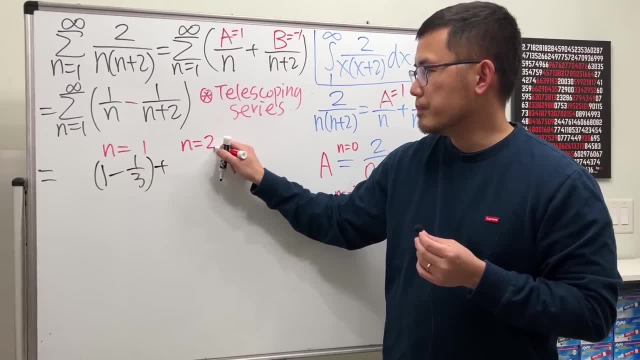 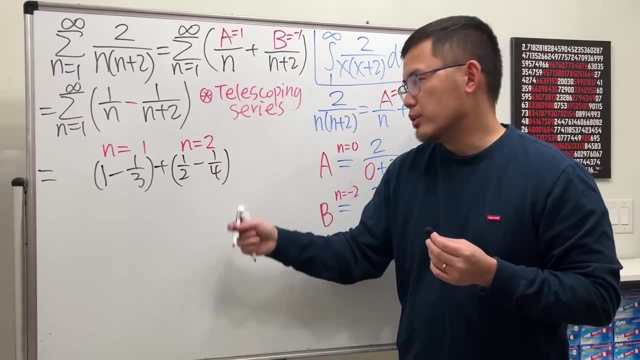 add the next term when we have n equals 2.. put 2 in here, and here we get 1 half minus 1 over 4.. continue, let's write down a few of them, plus the next one when n is equal to 3, and then you. 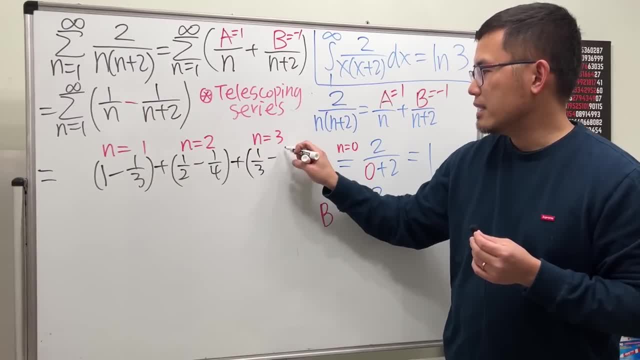 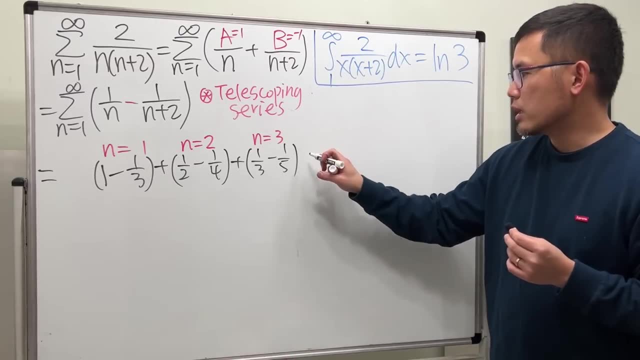 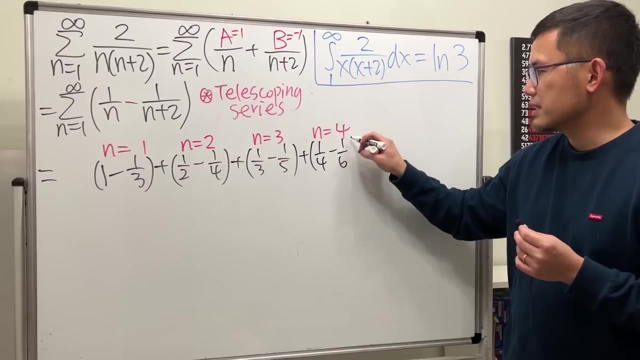 put 3 in here, and here we get 1 over 3 minus 1 over 5, and, of course, erase this and then continue. let's just put down one more term right here, that's when n equals 4, and that will give us 1 over 4 minus 1 over 6.. and now here's the deal: this and that they are off by two terms. 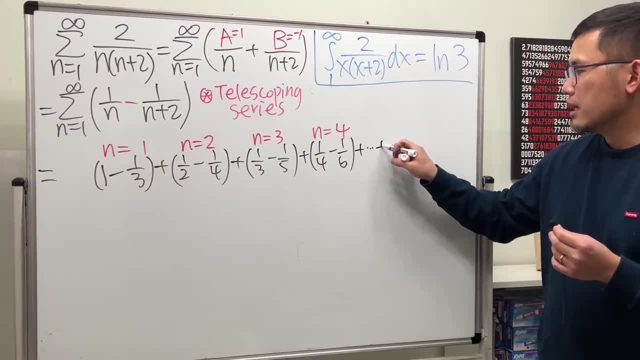 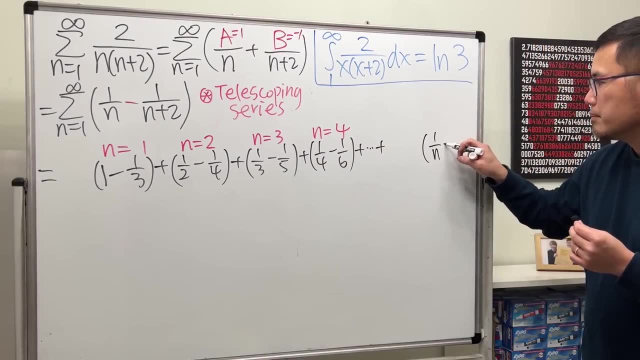 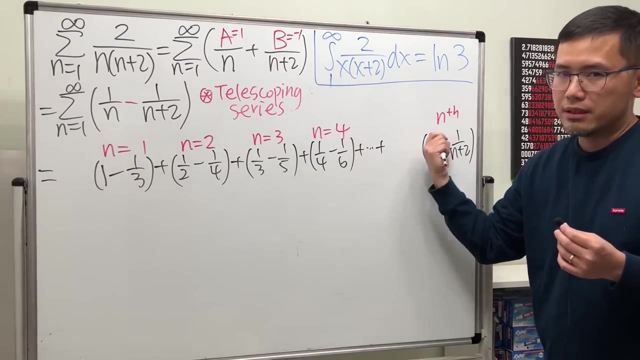 so i'm just going to put on plus dot, dot dot. i'm going to write down five vertices right here. the same thing. so that will be 1 over n minus 1 over n plus 2.. this right here is the nth term. when, when n is equal to n. yeah, but because this and that they are off by two terms. 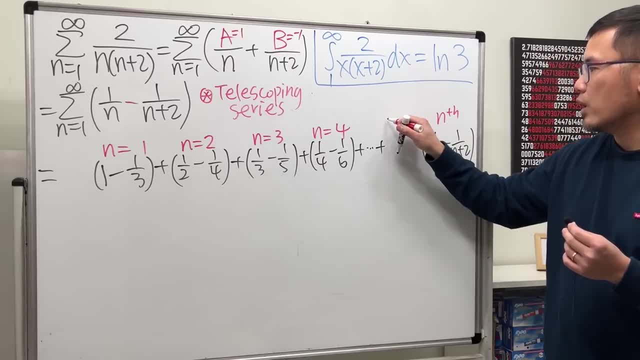 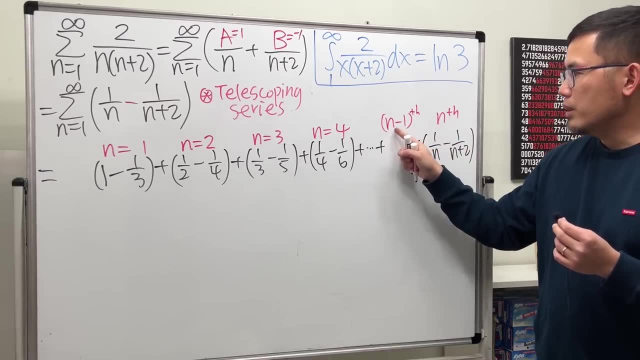 i need another one. i need its previous term as well, that's the n minus one term like this: so put n minus 1 into this n, we get 1 over n minus 1. and then let's also put a minus 1 in here. we just get 1 over n plus 1.. so that's minus 1 over n plus. 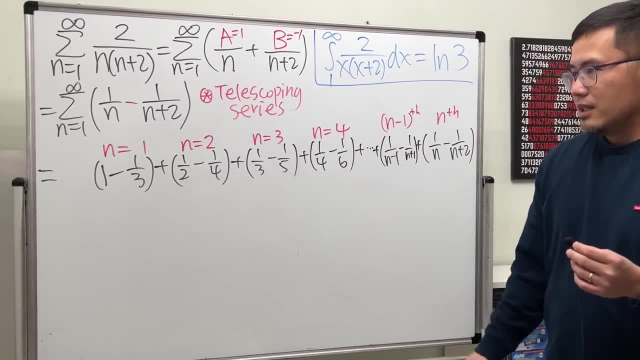 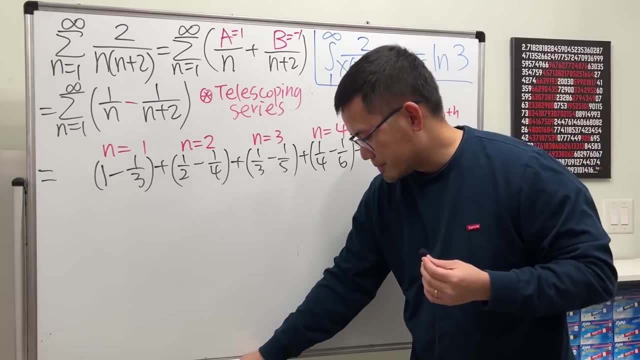 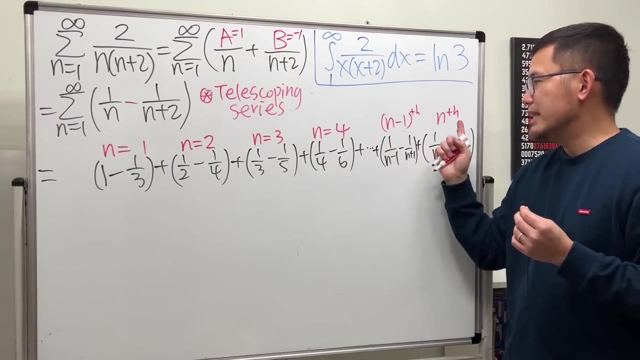 1. just like that. yeah, it's a long one, right, but don't worry, it's going to be clasping, right? you can put them back together. however, though- here's the deal, when you write them out this right, here is the nth partial sum. remember, when you are trying to. 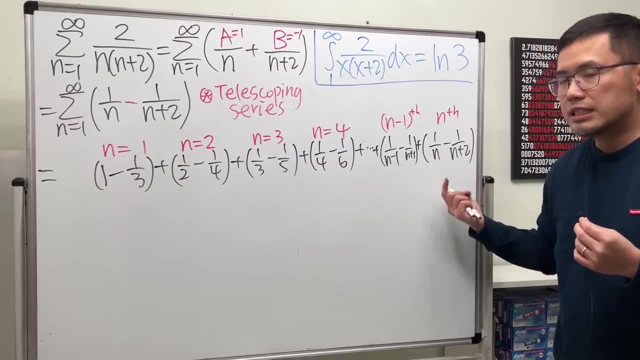 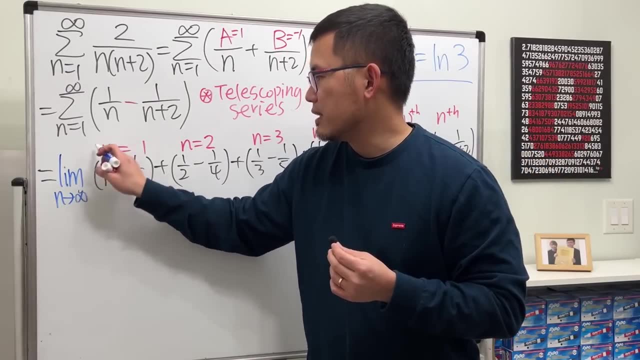 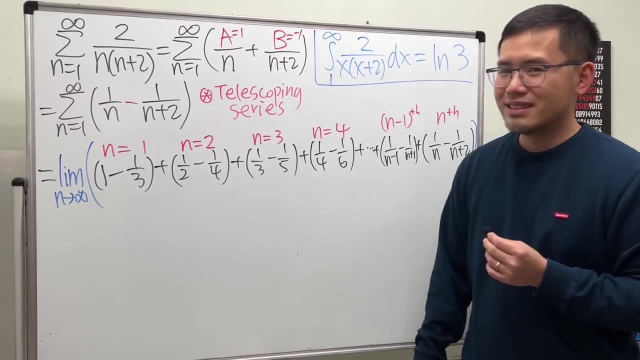 find the sum of infinite series. you can look at the nth partial sum and then take the limit. so here we will take the limit, as n goes to infinity of that. and now we can be really happy because good things are going to happen. have a look. first we have 1. 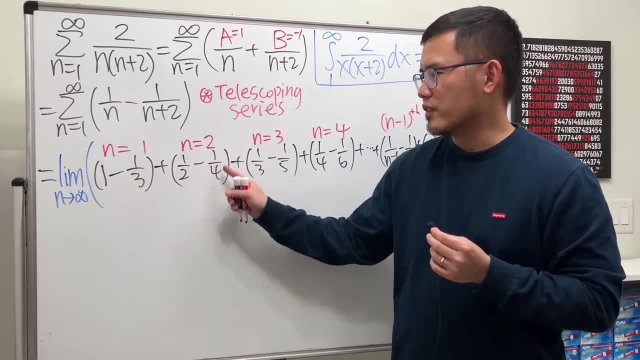 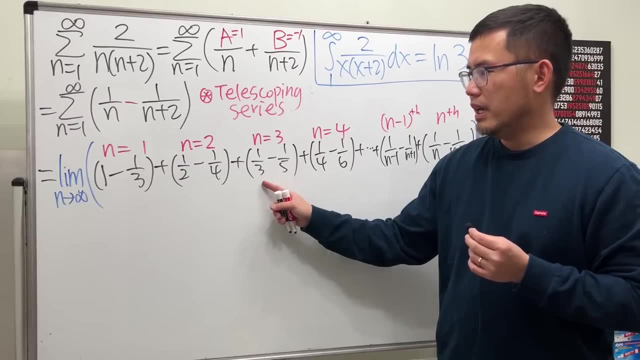 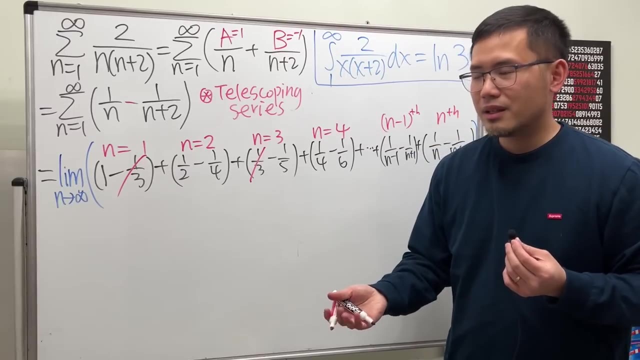 minus 1: 3.. 1 minus 1: 3.. plus one half. minus one over four. okay, and then next we have plus one over three. hey, we have a positive one over three, isn't this can be cancelled out with that, sure thing? yeah, and then continue. 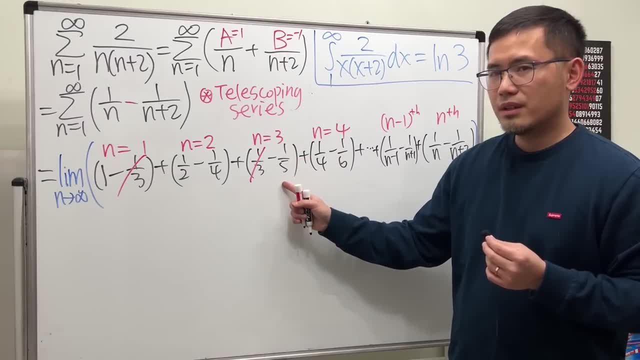 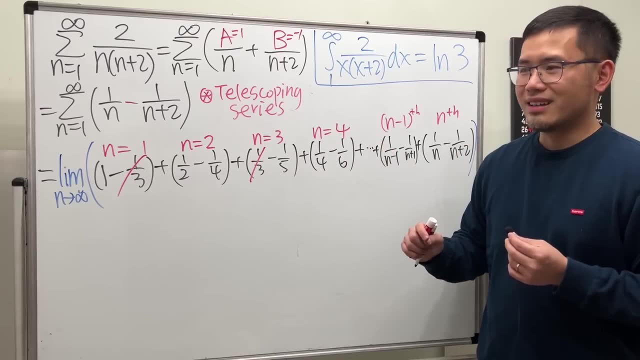 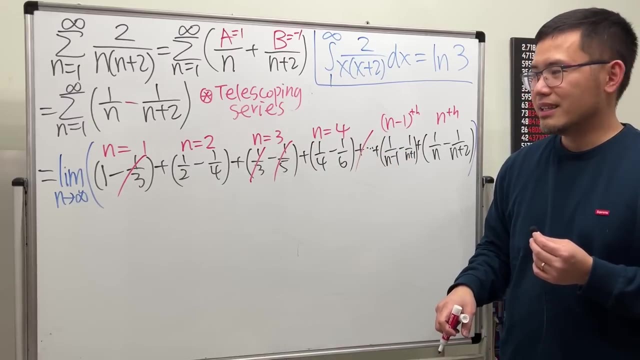 next one, we have minus one over five. but guess what? we can actually cancel this one as well with the one right here. i just didn't write it down. so imagine: if n is equal to five, then we can cancel this and that. yeah, and as you can see, 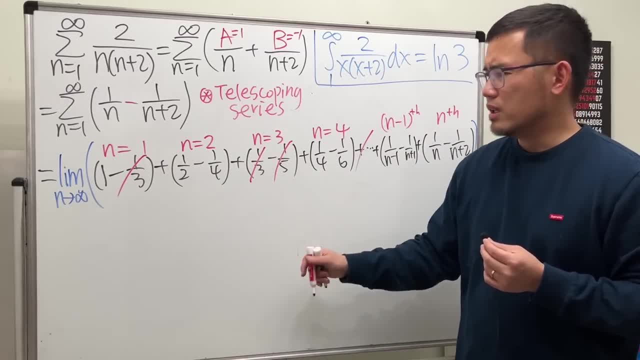 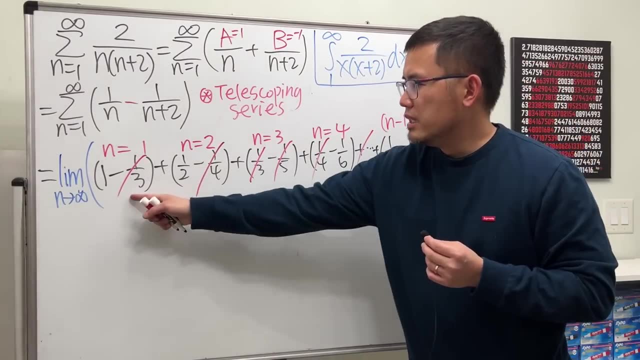 this right. here we have minus one over four and this is positive one over four, so we can cancel this. and that isn't it so far. we have one and one half remaining. this got cancelled with that. this got canceled. it was that this will be cancelled with that this. 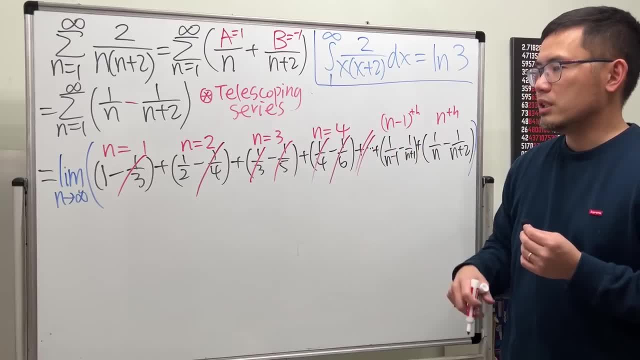 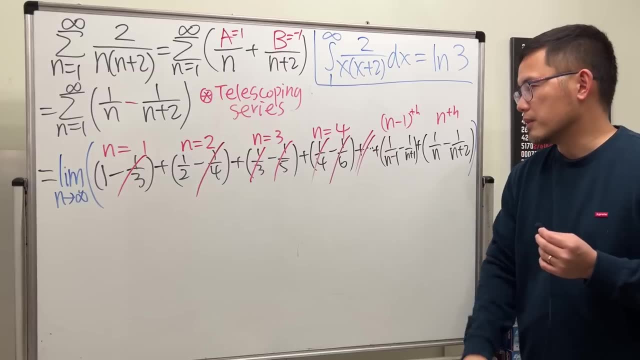 will be cancelled with something that we didn't write down by you. guys know what is the end of sqrt 3.. something that we didn't write down, but you know for sure it's going to be canceled. so a lot of these terms will be canceled. now be super, super careful. we have these two terms remaining, which. 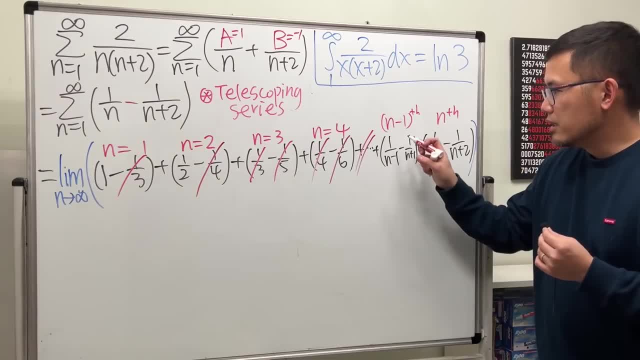 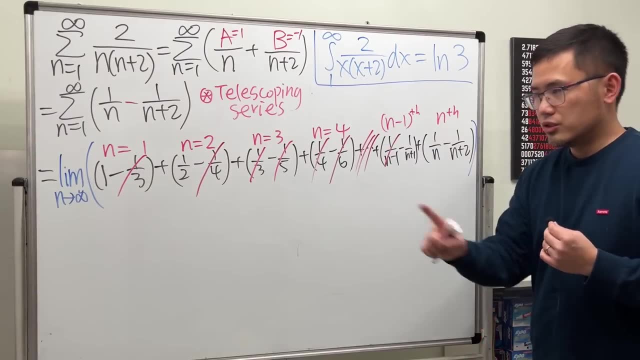 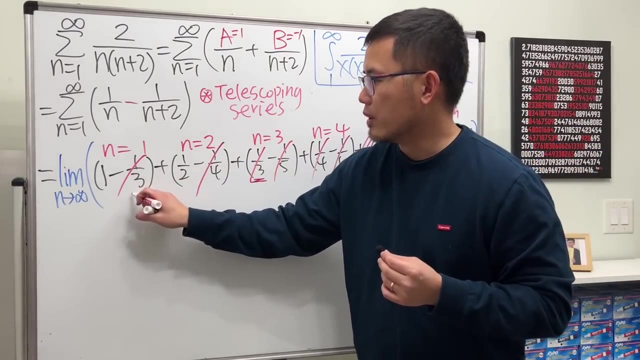 term will be canceled. the answer for that is the first term. this term- right here in this parentheses- will be canceled from the term. you know, two in the front, check this out. we had that one third here. right, this got canceled from, not this, but the term before. they got canceled, like that. 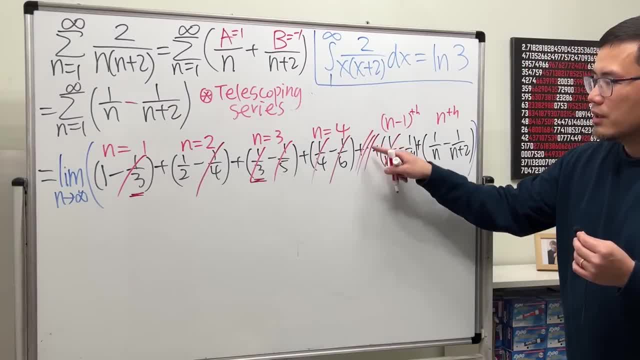 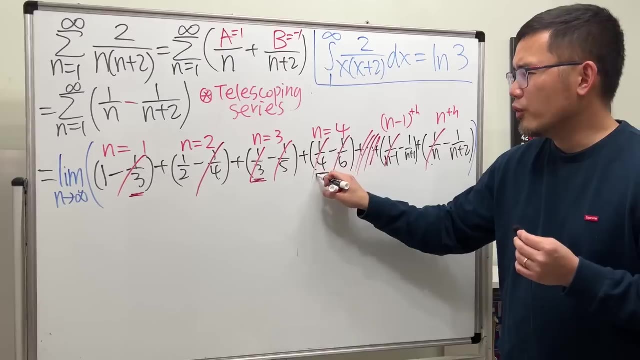 so this will be canceled from two terms before and then. if you take a look at this and that this term we also got canceled, not from here, but the term from its previous, so this will also be canceled here, just like when you see the one over four, you got canceled with this term. 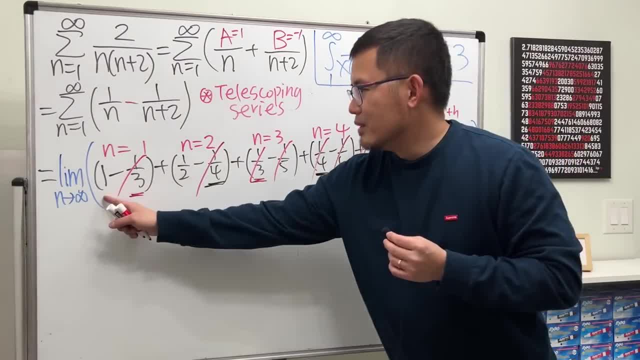 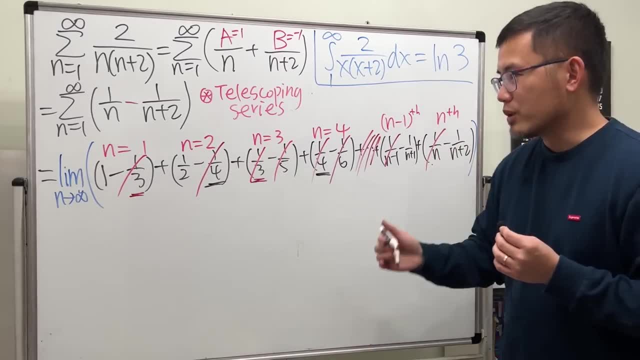 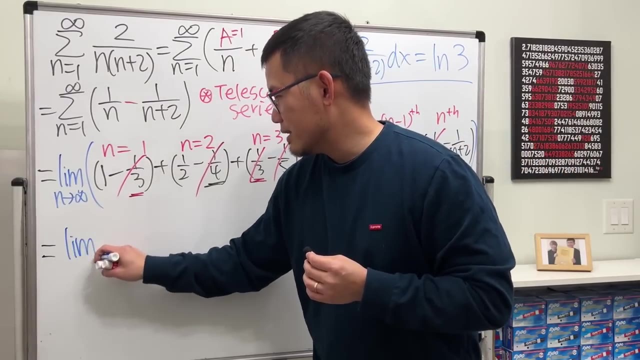 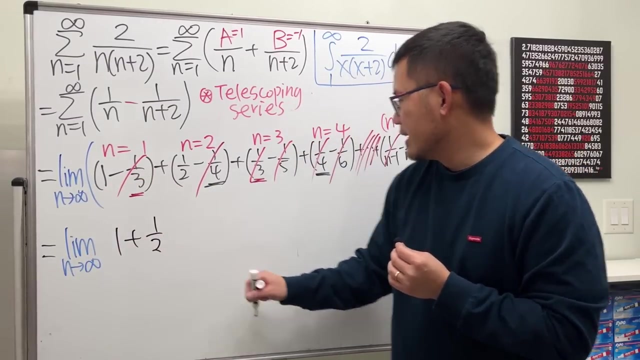 so we have one one plus one half, minus one over n plus one minus one over n plus two, these two, these four terms remaining. so here we have the limit. remember, still take the limit as n goes to infinity. we have one plus one half and then minus this. 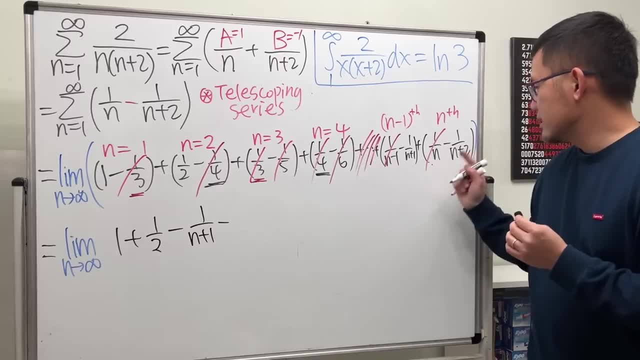 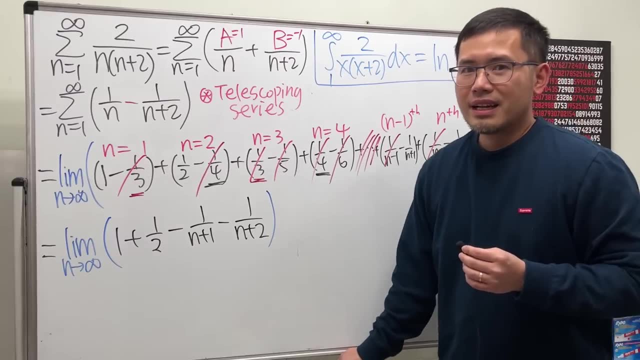 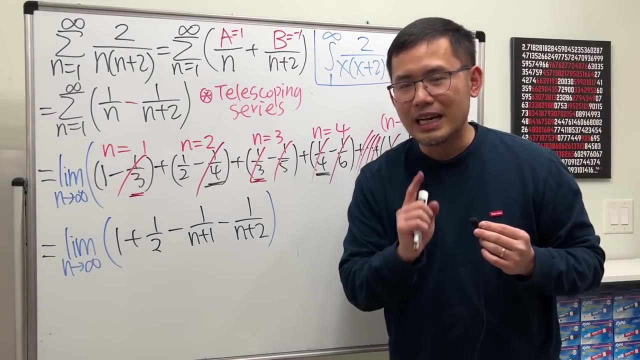 and then minus that, and then again. as i said, we'll take the limit for this now. here is the quick way to do this. you don't have to go through this every single time. this is how they are off by two terms. so what you do is you plug in. 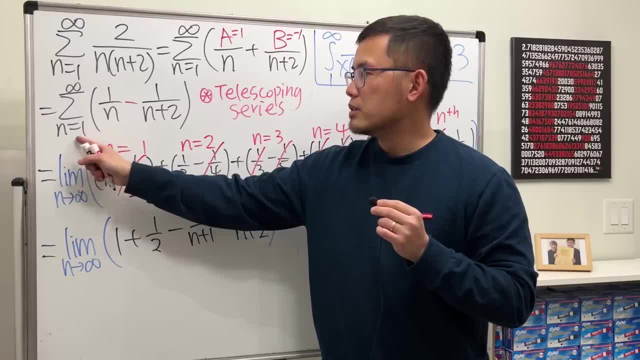 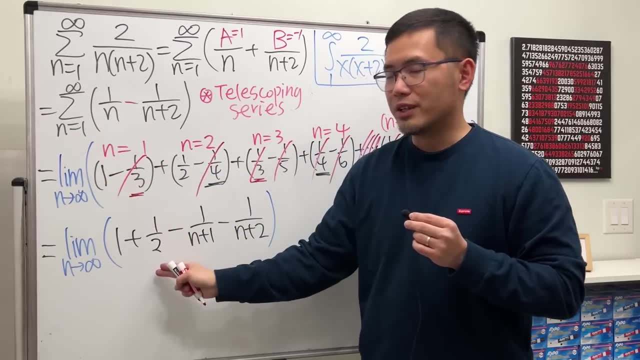 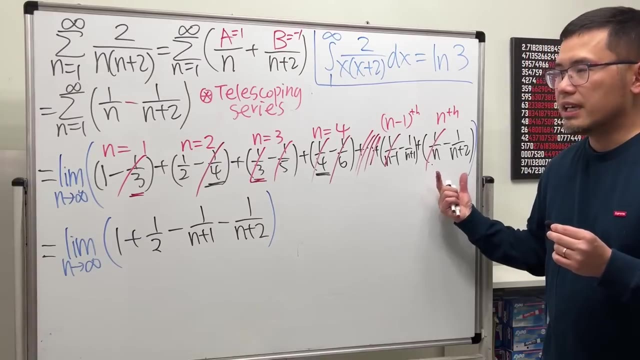 the starting value into the first turn here one time. so you get one over one right here, and then you do it again and it's equal to two. plug into here. only you get one over two. you need two terms in the front- okay done. and then you also need two terms at the end. so put down this term right here as how it is, and 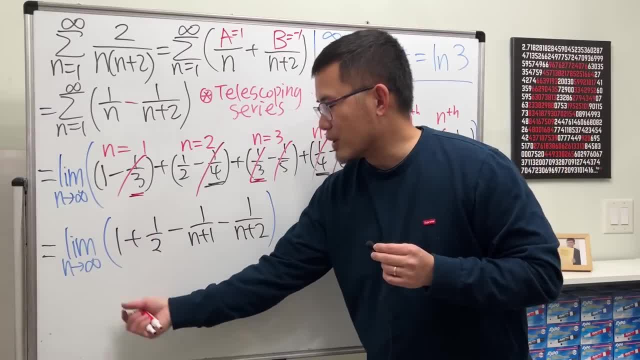 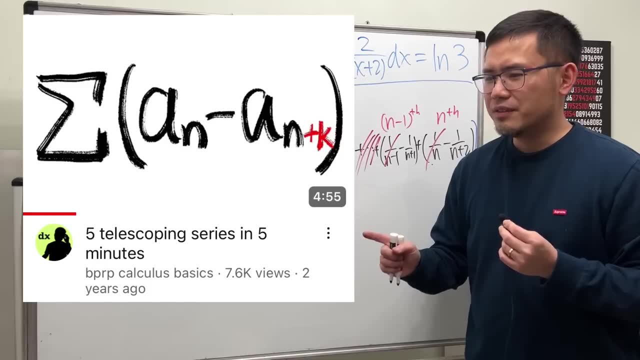 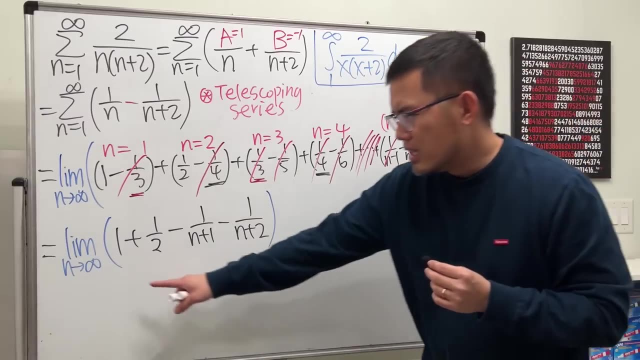 then its previous term, and you also subtract two terms in the front and then subtract two times in it at the end, because they're off by two. definitely check out my other video, because i showed you how to do the telescoping series like this very, very fast. but anyway, though n is approaching infinity. 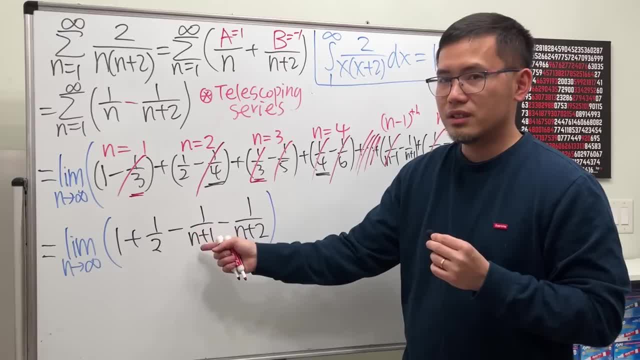 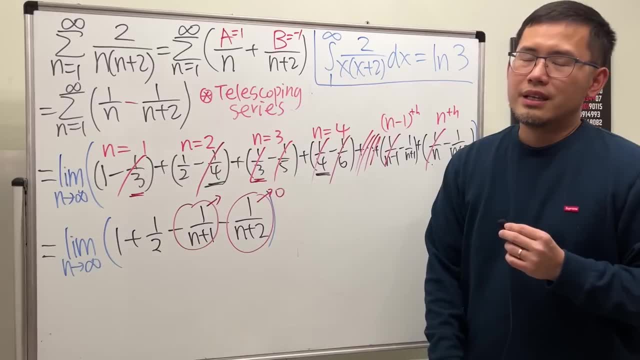 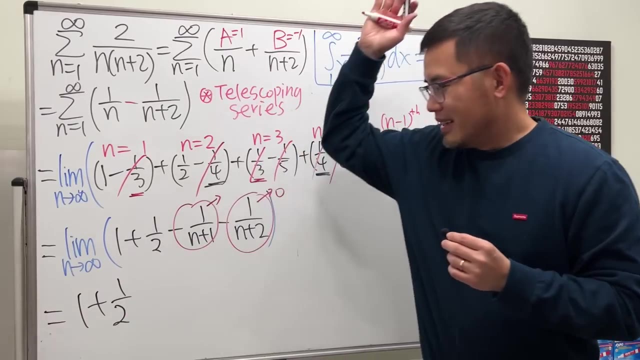 this term, we will just get one over infinity plus one, just infinity, which goes to zero. likewise, when you put infinity to here, this also goes to zero. so finally, we're just doing one plus one half and work out the fractions, you get three over two. yes, yeah. 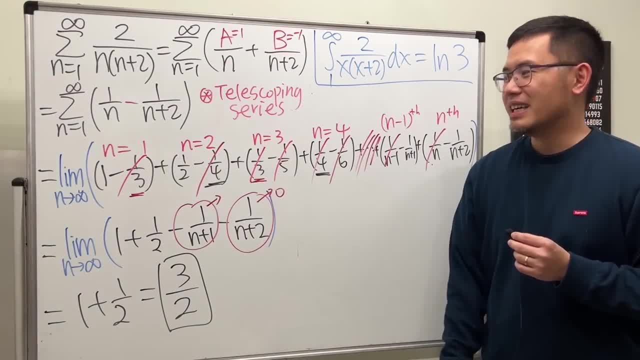 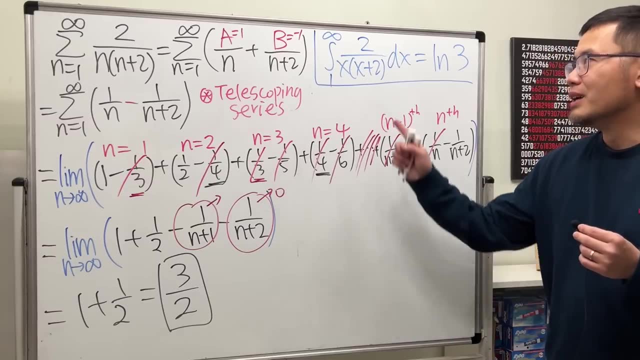 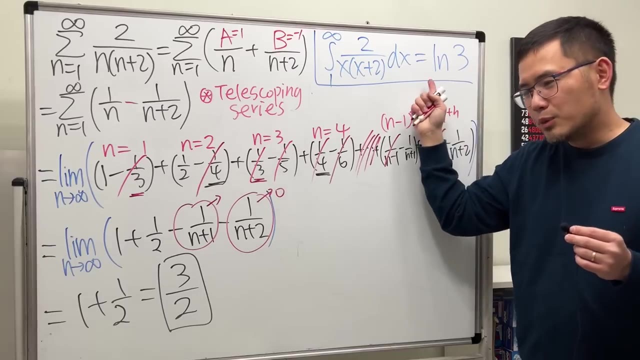 i've done a lot of this kind of questions, but every single time i do it, ah, it's just so wonderful. anyway, now, hopefully this right here helps. and don't forget: this is: try this on your own. make sure you know how to show. this is equal to ls3. if you need help with this, leave a comment down. 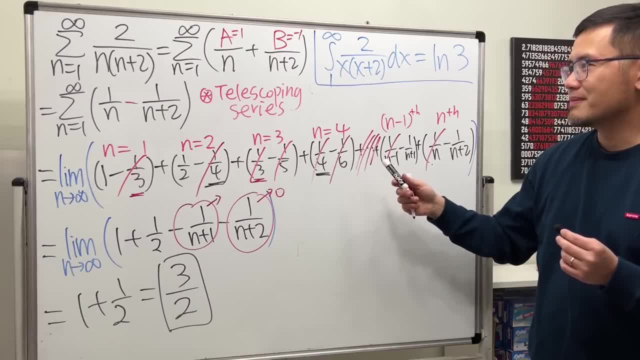 below, and let me know i'll make another video if i have time i will. i will anyway, though, that's it. 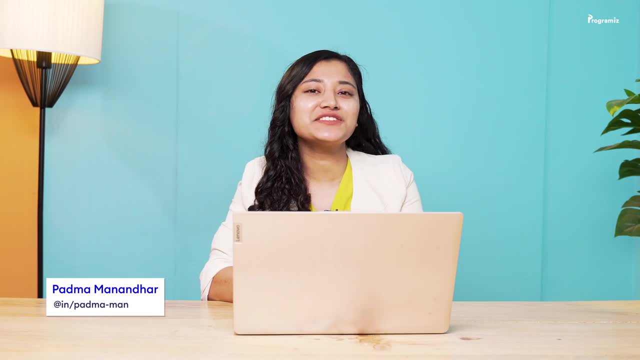 Hey guys, welcome back to this series on C programming. In the last video we learned about pointers. in C, We learned about working with memory addresses. Now we will learn to use pointers to work with arrays. So let's get started. 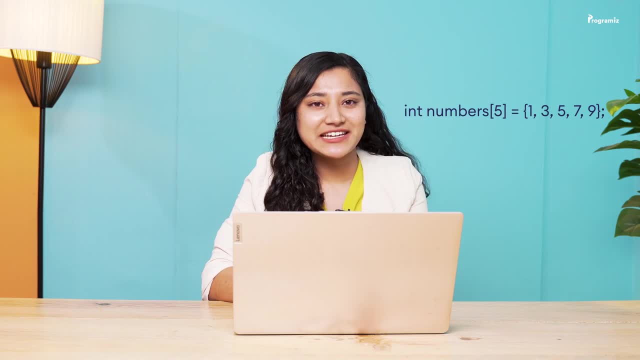 We know that an array is the collection of similar type of data. You can see the example on the screen Here: numbers is an array that stores 5 elements, And if we want to access these array elements, we can use the array index.